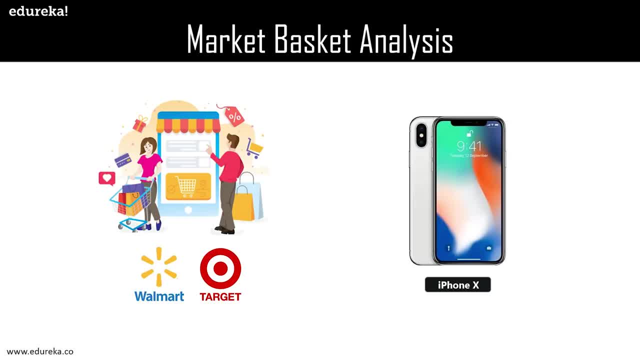 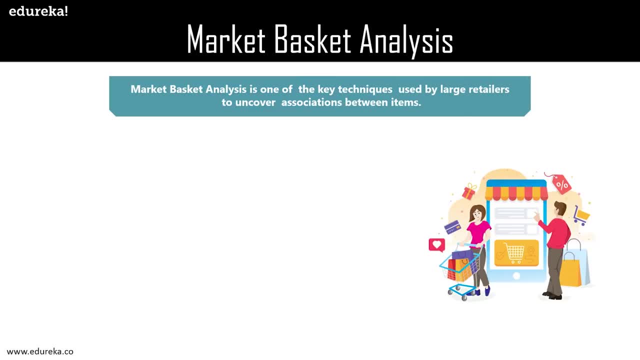 clearly no Hence organization began mining data relating to frequently bought items. So market basket analysis is one of the key techniques used by large retailers to uncover associations between items. Now examples could be: the customers who purchase bread have a 60% likelihood to also. 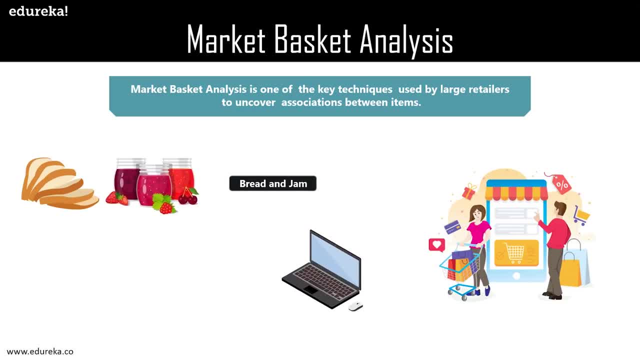 purchase jam. Customers who purchase laptops are more likely to purchase laptop bags as well. They try to find out associations between different items and products that can be sold together, which gives assisting in the right product placement. Typically it figures out what products are being bought together and organizations can place products in a similar. 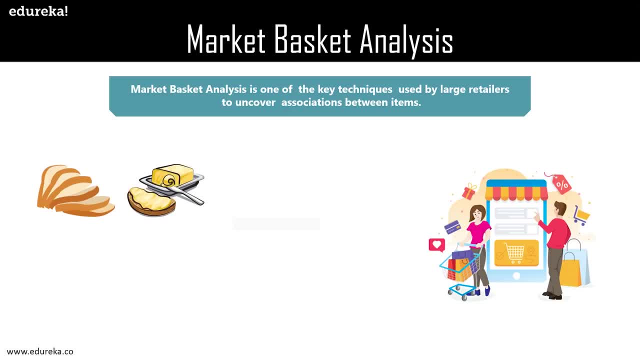 manner. For example, people who buy bread also tend to buy butter right, And the marketing team at retail stores should target customers who buy bread and butter and provide an offer to them so that they buy a third item, suppose eggs. So if a customer buys bread and butter and sees a discount, 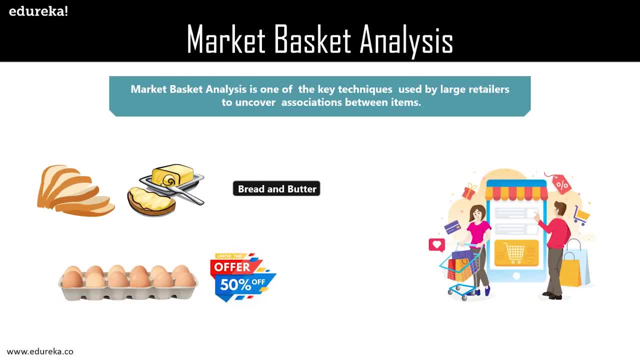 offer on eggs, he will be encouraged to spend more and buy the eggs, And this is what market basket analysis is all about. This is what we are going to talk about in this session, which is association rule, mulling and the a priori algorithm. Now association rule can be thought. 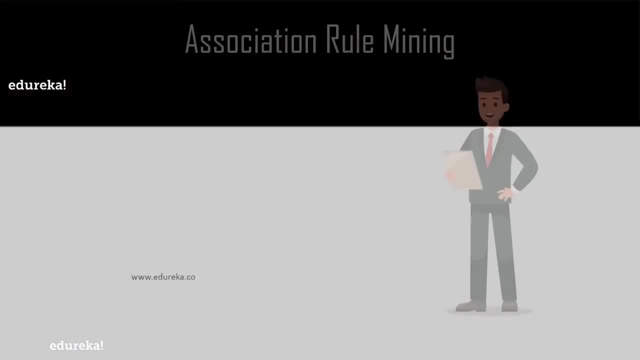 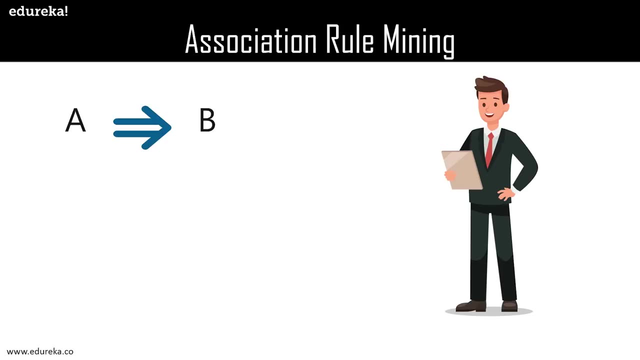 of as an if-then relationship. Just to elaborate on that, we have come up with a rule. Suppose if an item A is being bought by the customer, then the chances of item B being picked by the customer 2 under the same transaction ID, is found out. You need to understand here that it's not a casualty. 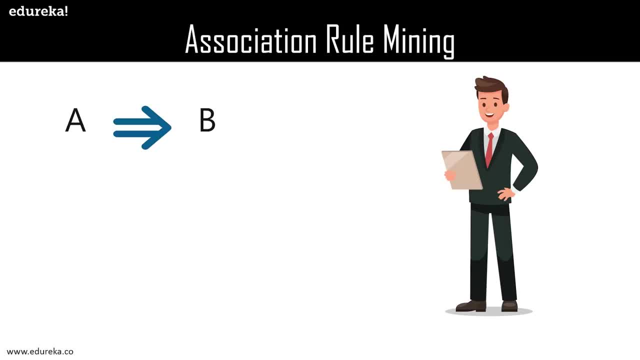 rather, it's a co-occurrence pattern that comes to the force. Now, there are two elements to this rule. First is the if and second is the then. Now if is also known as antecedent. This is an item or a group of items that are typically found in the item set And the later one. 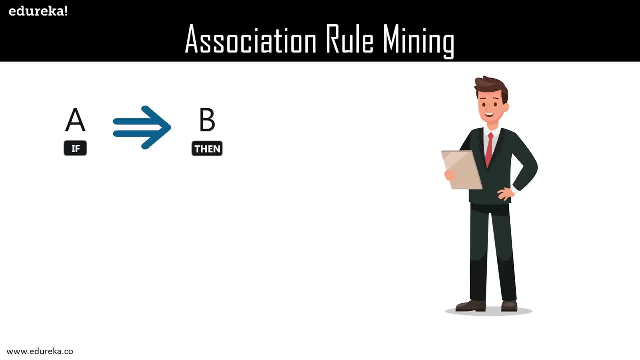 is called the consequent. This comes along as an item with an antecedent group, or the group of antecedents are purchased. Now, if you look at the image here, A arrow B, it means that if a person buys an item A, then he will also buy an item B. 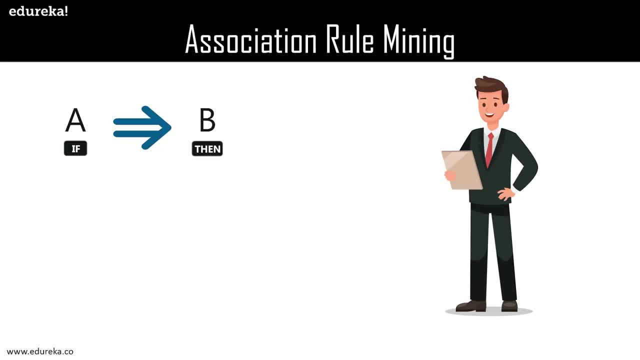 Or he will most probably buy an item B. Now, the simple example that I gave you about the bread and butter and the eggs is just a small example. But what if you have thousands and thousands of items? If you go to any professional data scientist with that data, you can just imagine how much of 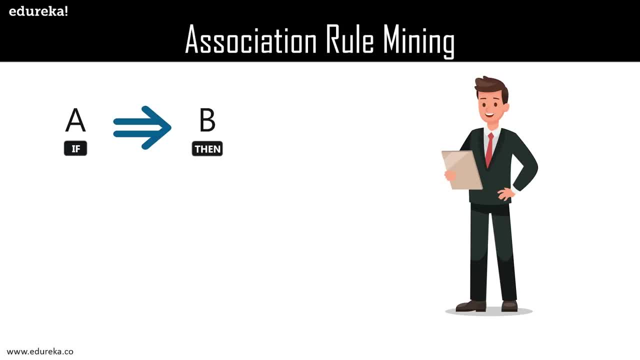 profit you can make if the data scientist provides you with the right examples and the right placement of the items, which you can do, And you can get a lot of insights. That is why association rule mining is a very good algorithm which helps the business make profit. So let's see how this algorithm works. 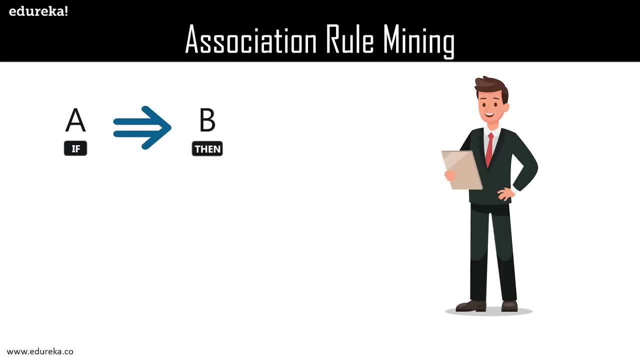 So association rule mining is all about building the rules, And we have just seen one rule that if you buy A, then there's a slight possibility or there's a chance that you might buy B also. This type of relationship, in which we can find the relationship between these two items, is known. 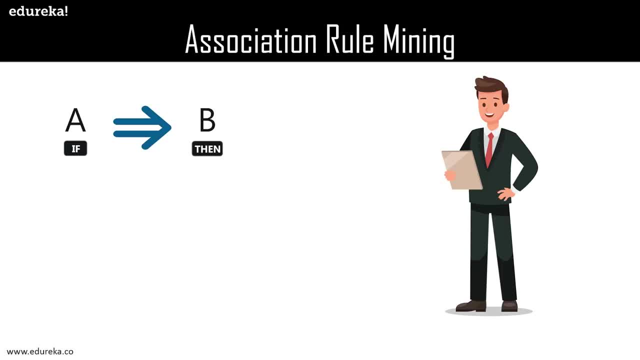 as single cardinality. But what if the customer who bought A and B also wants to buy C? Or if a customer who bought A, B and C also wants to buy D? Then in these cases the cardinality usually increases and we can have a lot of combination around these data. 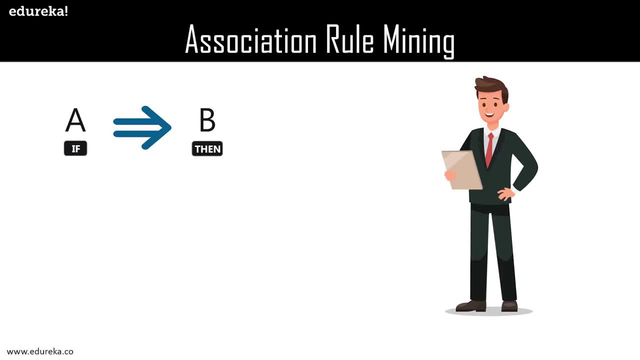 And if you have around 10,000 or more than 10,000 data or items, just imagine how many rules you're going to create for each product. That is why association rule mining has such measures, so that we do not end up creating tens of thousands of rules. Now that is where the a priori algorithm 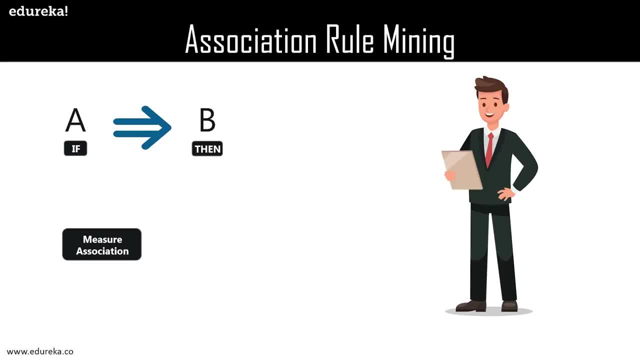 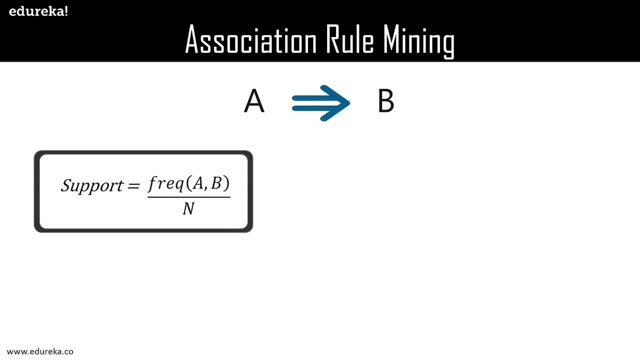 comes in. But before we get into the a priori algorithm, let's understand what's the maths behind it. Now there are three types of matrices which help to measure the association We have: support, confidence and lift. So support is the frequency of item A or the combination of item A. 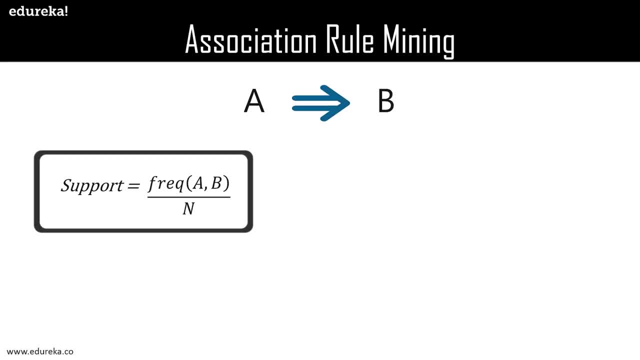 or B. It's basically the frequency of the items which we have bought and what are the combination of the frequency of the item we have bought. So with this, what we can do is filter out the items which have been bought less frequently. This is one of the measures which is support. 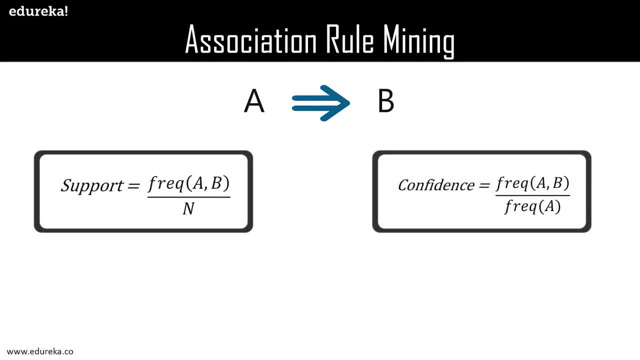 Now what confidence tells us? So confidence gives us how often the items A and B occur together, given the number of times A occur. Now this also helps us solve a lot of other problems, because if somebody is buying A and B together and not buying C, we can just rule out C at that point of time. 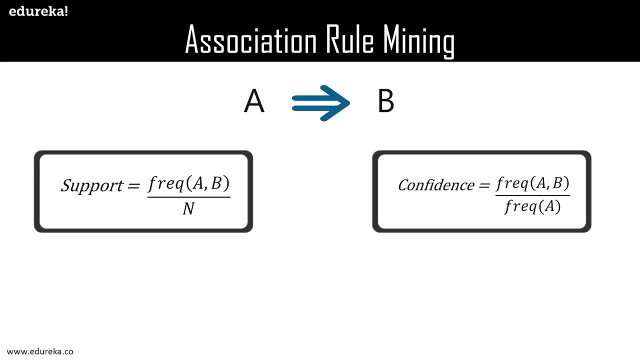 So this solves. another problem is that we obviously do not need to analyze the products which people just buy barely. So what we can do is, according to the sales, we can define our minimum support and confidence, And when you have set these values, we can put these values. 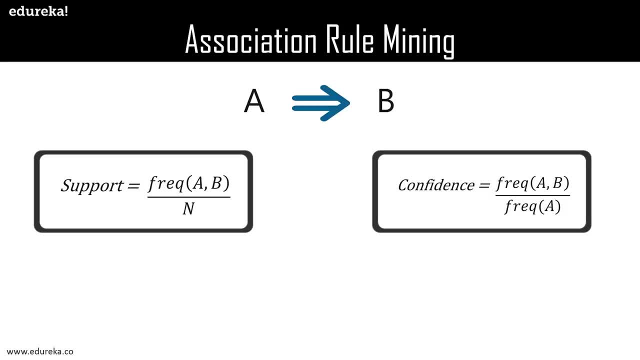 in the algorithm and we can filter out the data and we can create different rules. And suppose, even after filtering you have like five thousand rules and for every item we create these different rules. So that's practically impossible. So for that we need the third calculation. 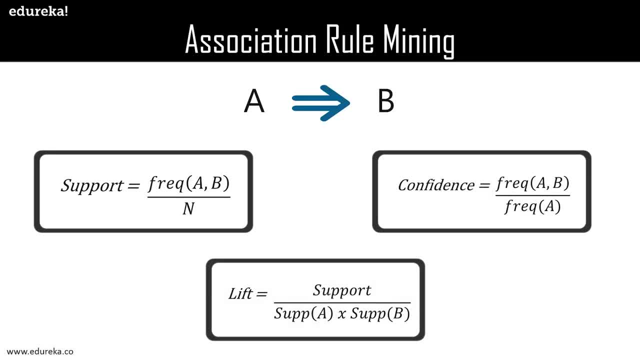 which is the lift. So lift is basically the strength of any rule. Now let's have a look at the denominator of the formula given here And if you see, here we have the independent support values of A and B. So this gives us the independent occurrence probability of A and B. 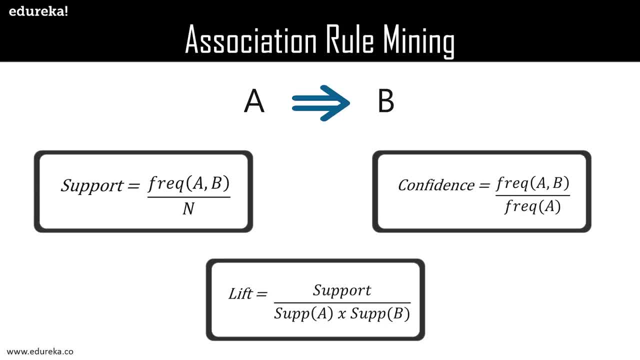 And obviously there's a lot of difference between the random occurrence and association. And if the denominator of the lift is more, what it means is that the occurrence of randomness is more rather than the occurrence because of any association. So lift is the final verdict where we know whether 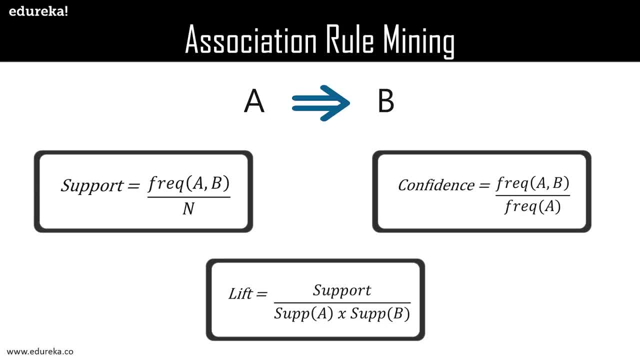 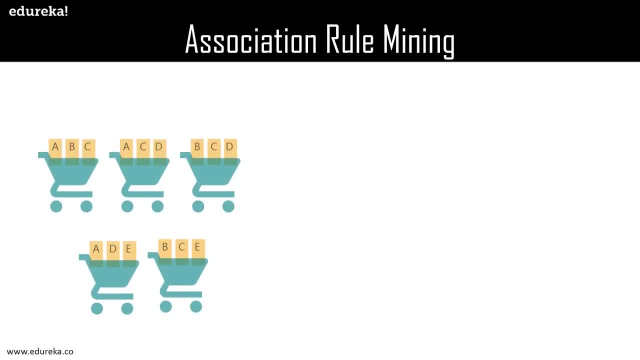 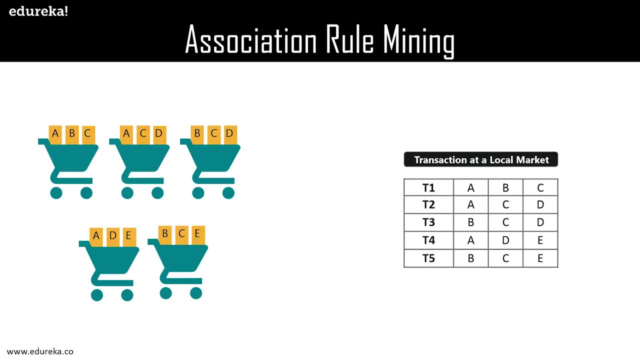 we have to spend time on this particular rule, what we have got here or not. Now let's have a look at a simple example of association rule mining. So suppose we have a set of items A, B, C, D and E and a set of transactions- T1, T2, T3, T4 and T5. And, as you can see, here we have the 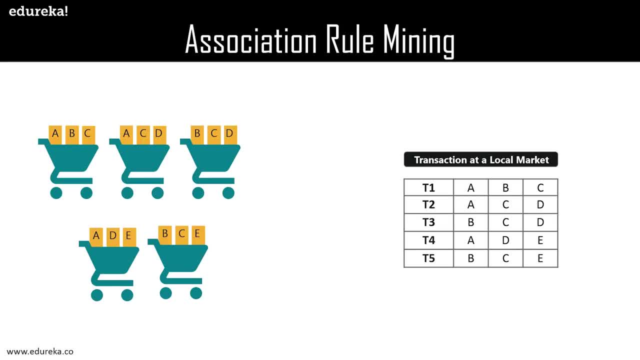 transactions T1, in which we have A, B, C, T2, A C D, T3, B C, D, T4, A D, E and T5, B C- E. Now what we generally do is create some rules or association rules, such as A gives T or C gives A. 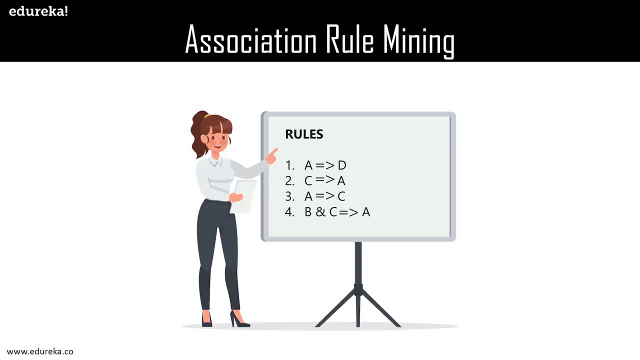 A gives C, B and C gives A. What this basically means is that if a person buys A, then he is most likely to buy D, And if a person buys C, then he is most likely to buy A. If you have a look at the last one, if a person buys B and C is most likely to buy the. 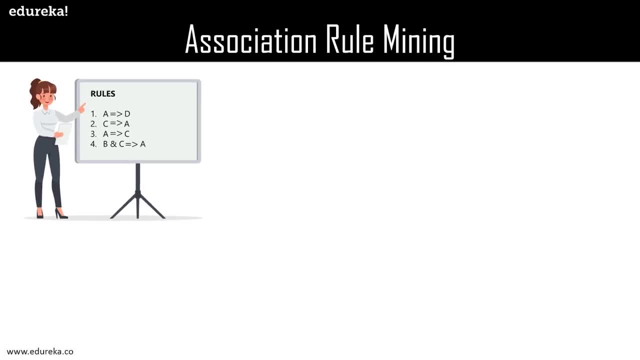 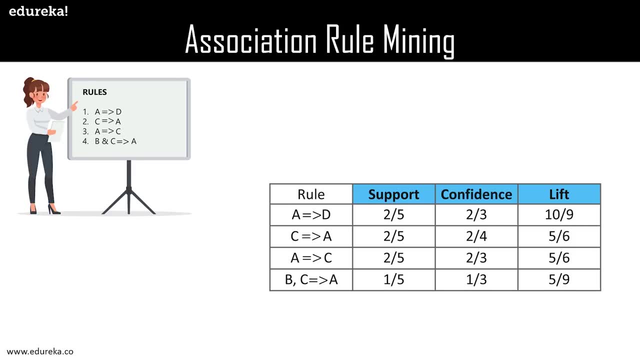 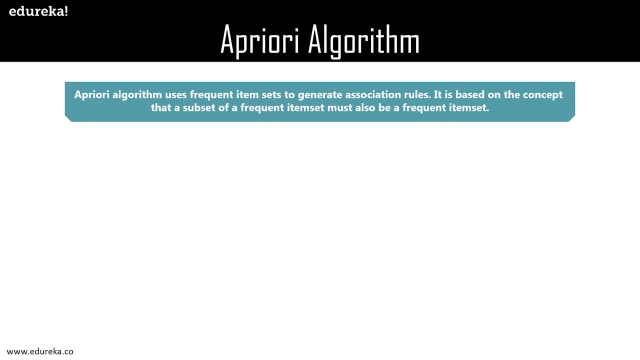 item A as well. Now, if we calculate the support confidence and lift using these rules, as you can see here in the table, we have the rule and the support confidence and the left values. Now let's discuss about PRIORITY. So PRIORITY algorithm uses the frequent item. 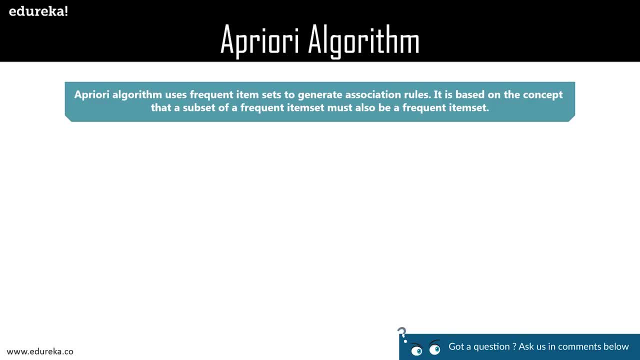 sets to generate the association or intrinsic value for A rule, and it is based on the concept that a subset of a frequent item set must also be a frequent item set itself. now this raises the question: what exactly is a frequent item set so a frequent item? 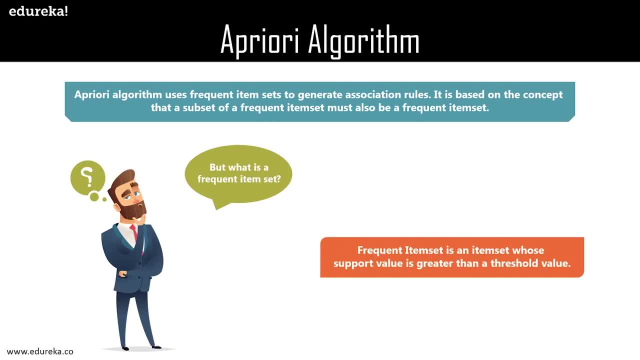 set is an item set whose support value is greater than the threshold value. now, just now we discussed that the marketing team, according to the sales, have a minimum threshold value for the confidence as well as the support so frequent items up. is that a them set who support value is greater than? 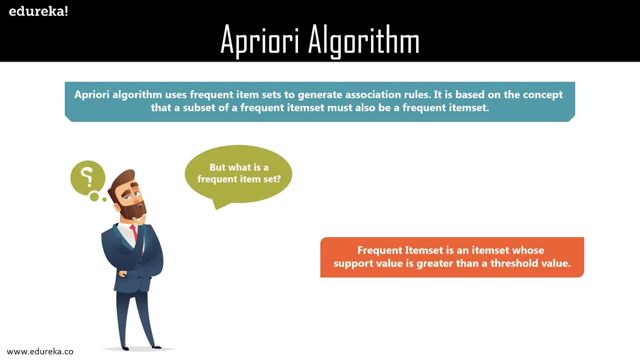 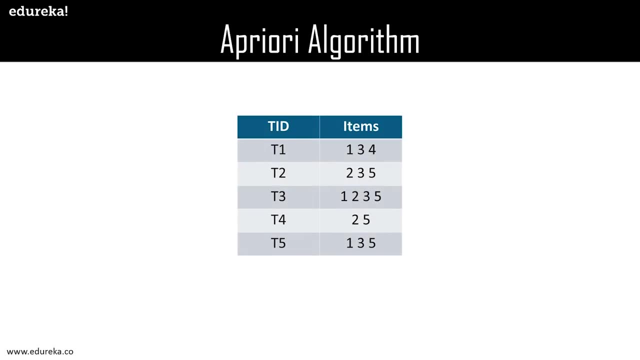 the threshold value already specified the example. if a and B's a frequent item set, then a and B should also be frequent item sets individually. now let's consider the find transaction. to make the things a little easier, suppose we have transactions one, two, three, four, five and these: 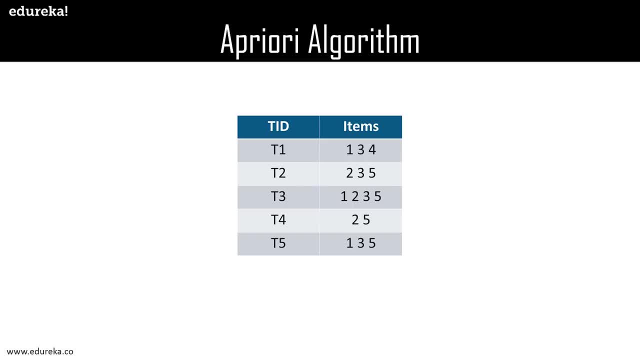 items are there. so t1 has one, three and four, t2 has two, three and five, T three has one and five and T three has four and five. so the following process is a frequent item set: 1, 2, 3, 5, t 4, 2, 5 and t 5, 1, 3 and 5. now the fourth step is to build a list of item sets of size 1. 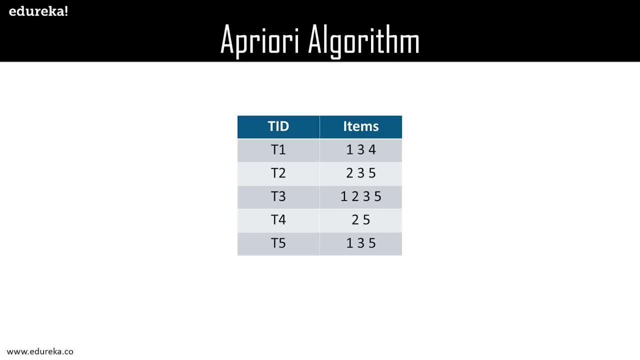 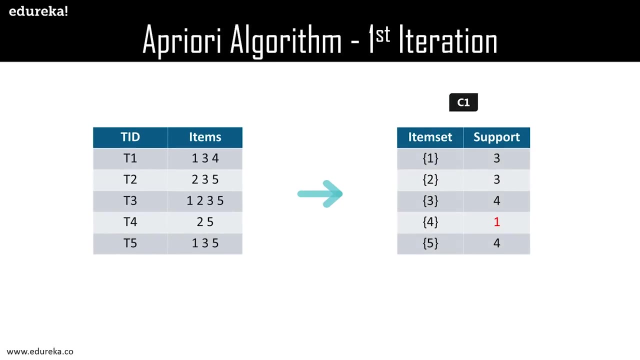 by using this transactional data. and one thing to note here is that the minimum support count which is given here is 2- let's suppose it's 2- so the first step is to create item sets of size 1 and calculate their support values. so, as you can see, here we have the table c1, in which we have 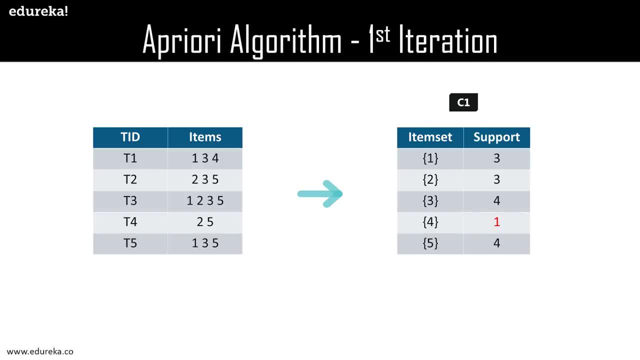 the item sets 1, 2, 3, 4, 5 and the support values. if you remember the formula of support, it was frequency divided by the total number of occurrence. so as you can see here, for the item set 1 the support is 3. as you can see here, that item set 1 appears in t1, t3 and t5. so as you can see its 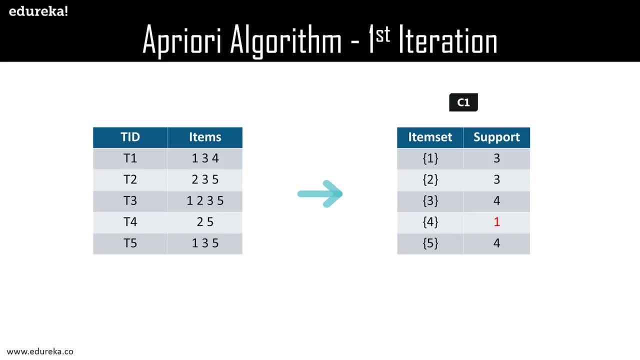 frequency is 1, 2 and 3. now, as you can see here the item set, 4 has a support of 1, as it occurs only once in transaction 1, but the minimum support count is 3. so, as you can see here the item set, 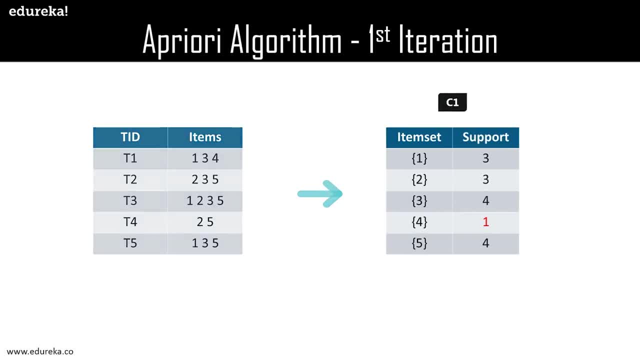 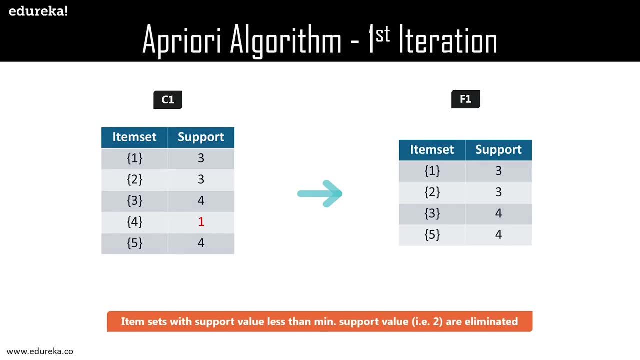 4 has a support of 1, as it occurs only once in transaction- 1, but the minimum support value is 2. that's why it's going to be eliminated. so we have that final table, which is the table f1, in which we have the item sets 1, 2, 3 and 5 and we have the support values 3, 3, 4 and 4. now the next. 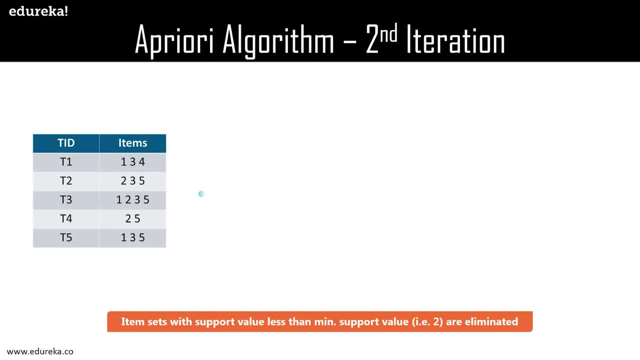 step is to create item sets of size 2 and calculate their support values. now, all the combination of the item sets in the f1, which is the final table in which we discarded the 4, are going to be used for this iteration, so we get the table c2. 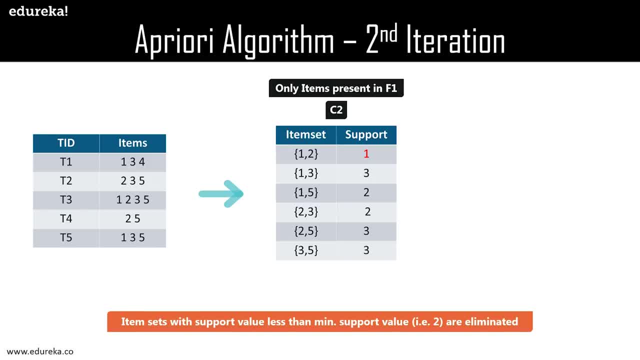 so as you can see, here we have 1, 2, 1, 3, 1, 5, 2, 3, 2, 5 and 3, 5. now if you calculate the support here again, we can see that the item set 1 comma 2 has a support of 1, which is again less than the. 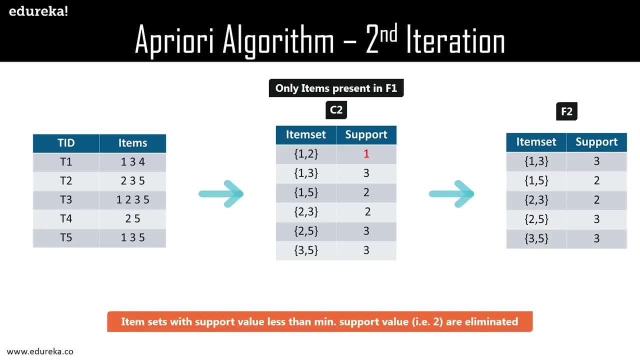 specified threshold. so we're going to discard that. so if we have a look at the table f2, we have 1 comma, 3, 1, 5, 2, 3, 2, 5 and 3, 5. again. we're going to move forward and create the item set of size 3. and calculate the support value of the item set 1, 2, 3, 1, 5, 2, 3, 2, 5 and 3, 5. again we're going to move forward and create the item set of size 3 and calculate the support values. now all the. 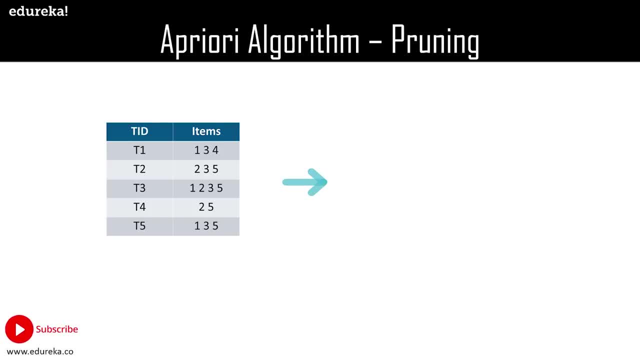 combinations are going to be used from the item set f2 for this particular iterations. now, before calculating support values, let's perform pruning on the data set. now, what is pruning? now, after the combinations are being made, we divide c3 item sets to check if there is another subset whose support 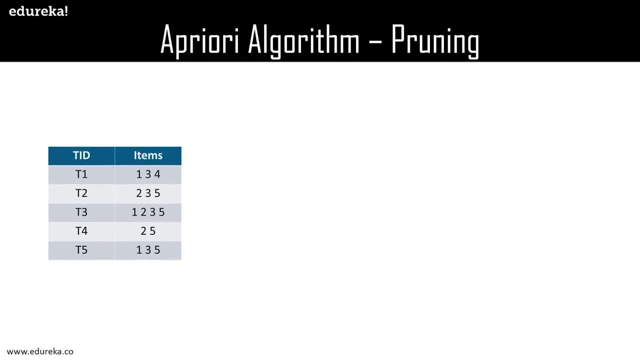 is less than the minimum support value. that is what frequent item set means. so if we have a look here, the item sets we have is 1, 2, 3 and 4 and 5 and 6 and 7 and 8 and 9 and 10 and 11 and 12 and 11 and. 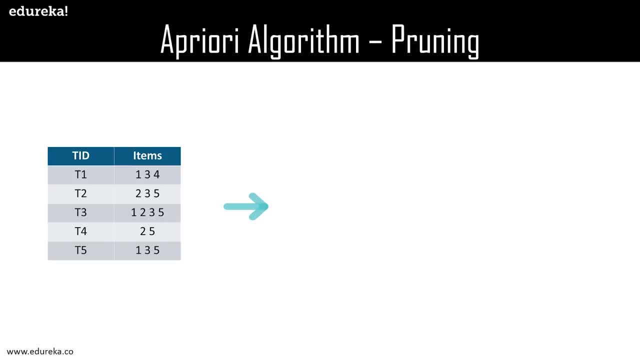 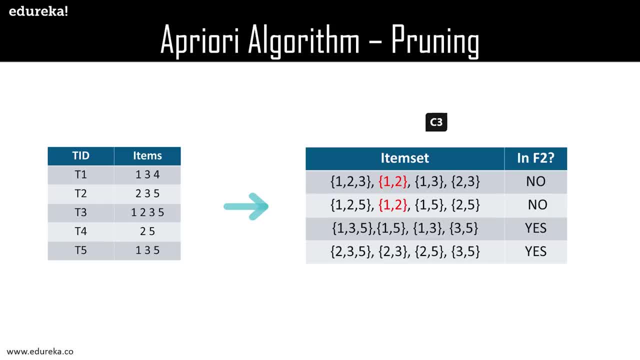 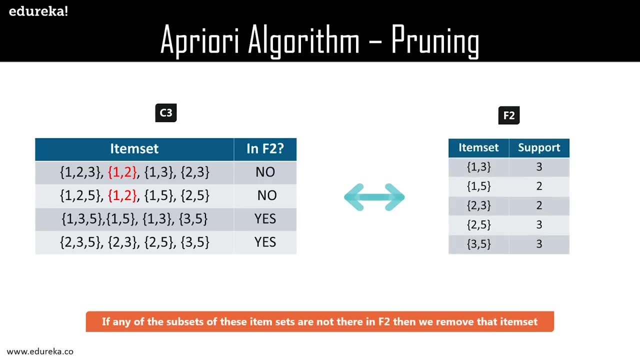 we are going to discard this whole item set. same goes for the second one. we have 1, 2, 5. we have 1, 2 in that which was discarded in the previous set or the previous step. that's why we're going to discard that also, which leaves us with only two factors, which is 1, 3, 5 item set and the 2, 3, 5. so 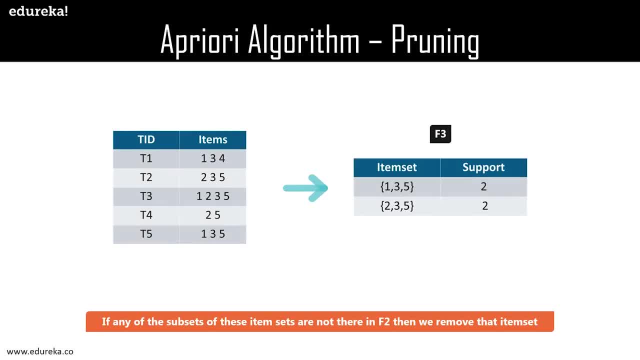 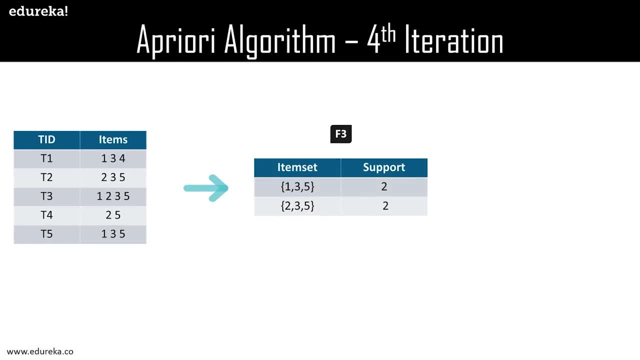 a support for this is 2 & 2 as well. now, if we create the table C 4 using 4 elements, we're gonna have only one item set, which is 1, 2, 3 & 5, and if we have a look at the table here- the transaction table- 1, 2, 3 & 5- appears only 1. so the 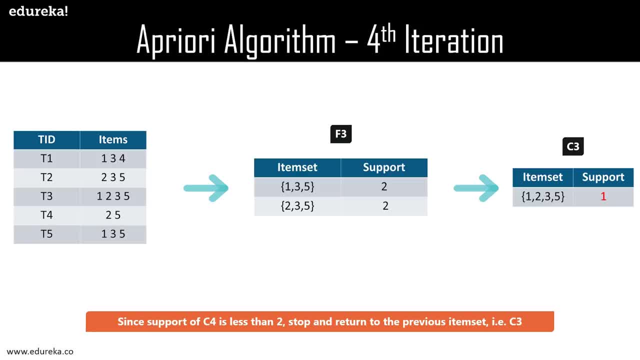 support is 1 and since C 4- the support of the whole table C 4- is less than 2. so we're gonna stop here and return to the previous item set, that is C 3. so the frequent item sets are 1, 3, 5 & 2, 3, 5. now let's assume our minimum confidence. 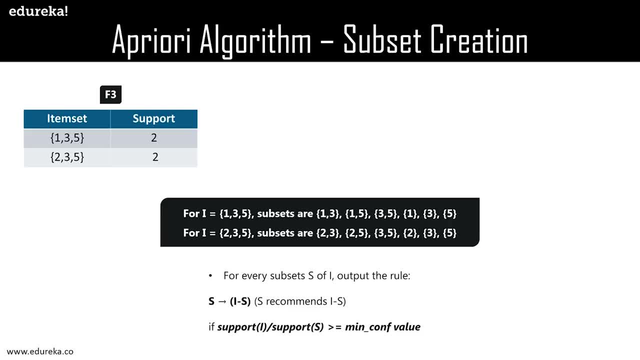 value is 60%. for that we're going to generate all the non empty subsets for each frequent item sets. now for I equals 1, comma 3, comma 5, which is the item set, we get the subset 1, 3, 1, 5, 3, 5, 1, 3 & 5. similarly, for 2, 3, 5, we get 2, 3, 2, 5, 3, 5, 2. 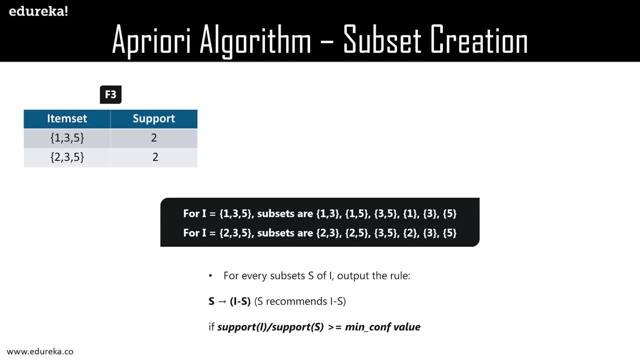 3 & 5. now this is the same item set that we created earlier. now, if we get the subset 1, 3, 1, 5, 5, this rule states that for every subset s of i, the output of the rule gives something like s. gives i to s. that implies s. 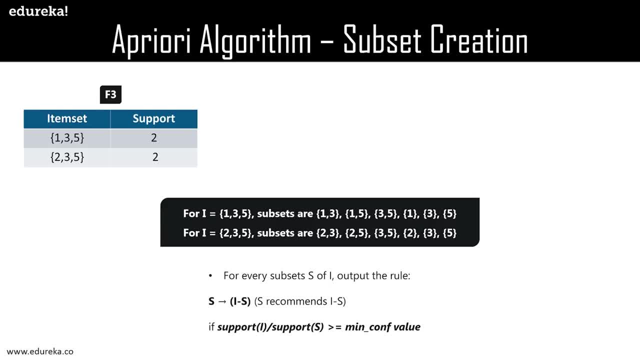 recommends i of s, and this is only possible if the support of i divided by the support of s is greater than equal to the minimum confidence value. now, applying these rules to the item set of f3, we get rule 1, which is 1. 3 gives 1. 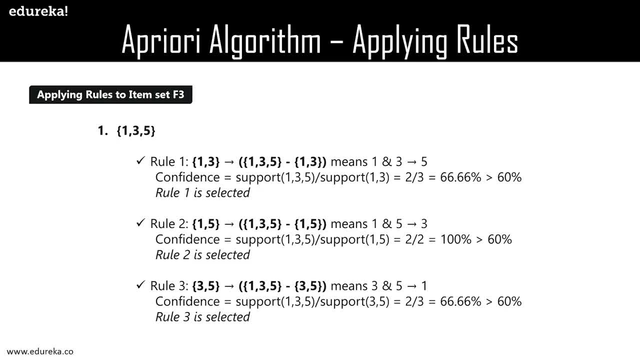 comma 3, comma 5 & 1- 3. it means 1, 3 is the minimum confidence value of the whole. it means 1 and 3 gives 5. so the confidence is equal to the support of 1 comma, 3, comma 5. 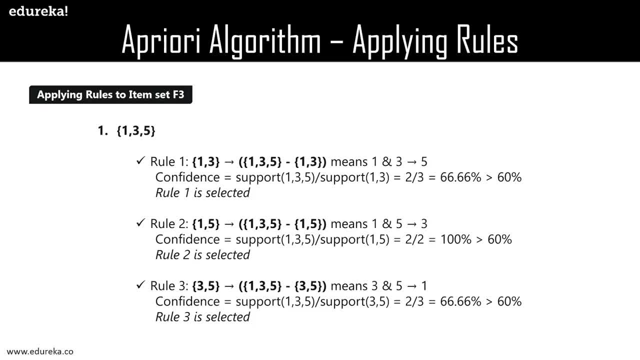 divided by the support of 1 comma 3, that equals 2 by 3, which is 66 percent, and which is greater than the 60 percent. so the rule 1 is selected. now, if we come to rule 2, which is 1 comma 5, 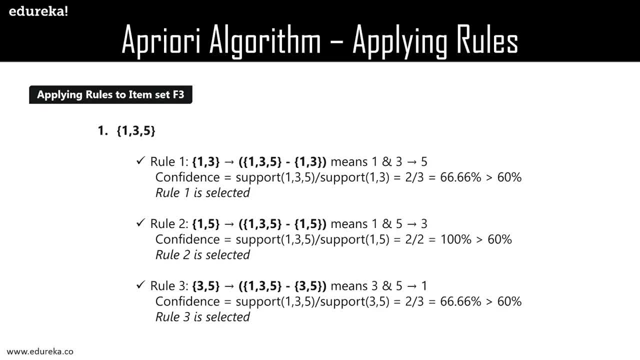 it gives 1 comma, 3 comma 5 and 1- 5. it means if we have 1 and 5, it implies we also going to have 3.. now if we calculate the confidence of this one, we're going to have support 1, 3, 5 divided by 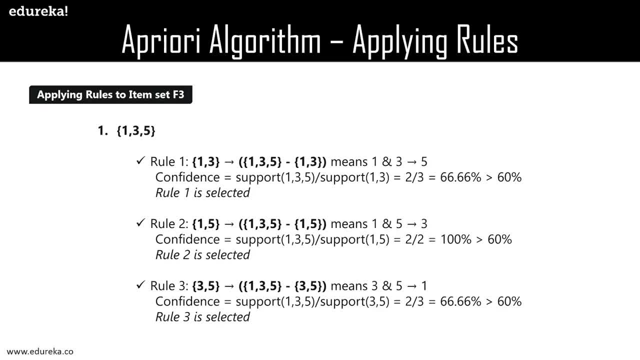 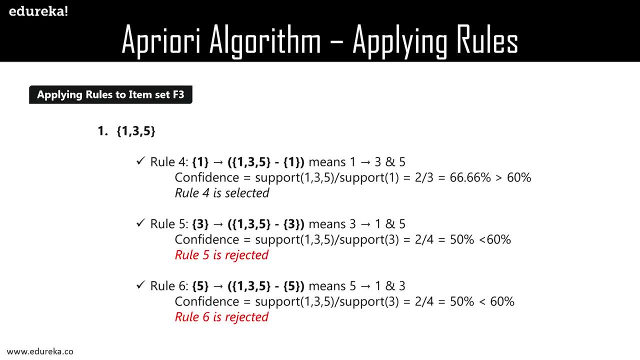 support 1- 5, which gives us 100 percent, which means rule 2 is selected as well. but again, if we have a look at rule five and rule six over here, similarly if we select three gives one, three, five and three. it means if we have three we also get one and five. so the confidence for this comes at. 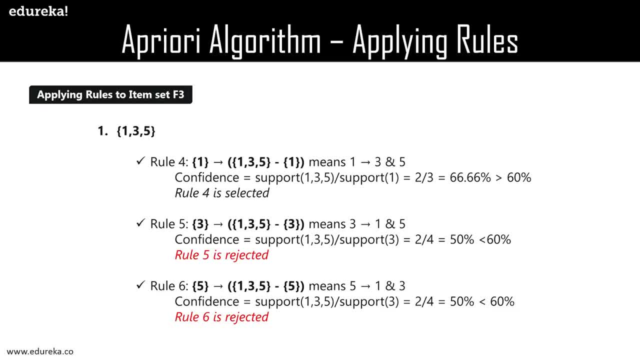 fifty percent, which is less than the given sixty percent target. so we're going to reject this rule, and so same goes for the rule number six. now, one thing to keep in mind here is that although the rule one and rule five look a lot similar, they are not. so it really depends what's on the left hand side of 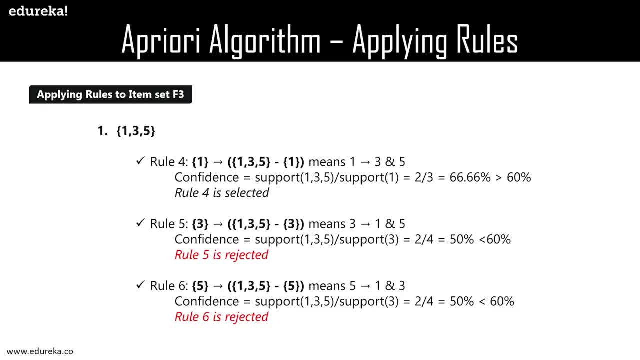 the arrow and what's on the right hand side of the arrow? it's the if, then possibility. i'm sure you guys can understand what exactly these rules are and how to proceed with these rules. so let's see how we can implement the same in python, right? so for that, what i'm going to do is create a new. 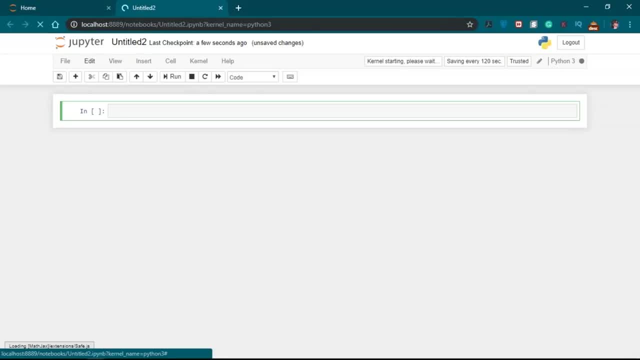 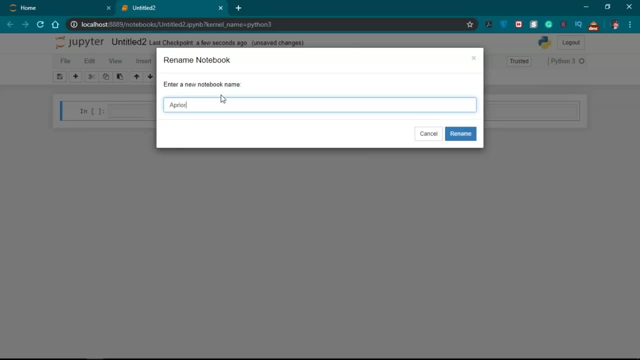 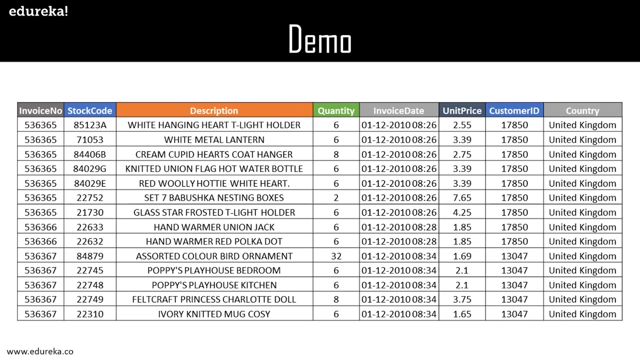 python file and i'm going to use the jupyter notebook. you're free to use any sort of id. i'm going to name it as a priority. so the first thing, what we're going to do is we'll be using the online transactional data of retail store for generating association rules. 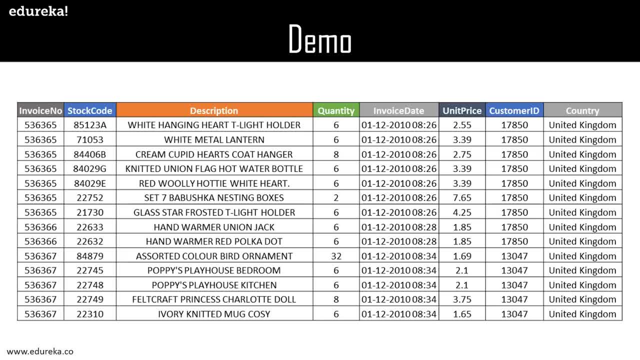 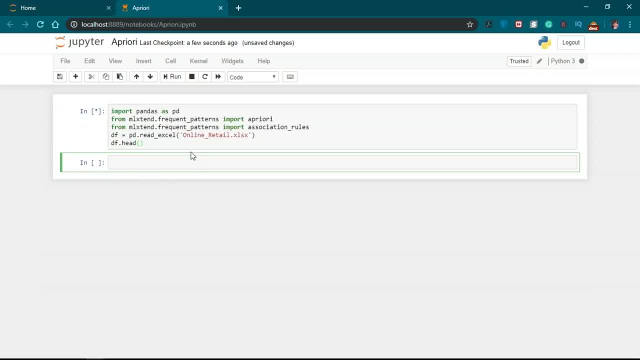 so, firstly, what we need to do is get the pandas and mlxtel libraries imported and read the file. so, as you can see, here we are using the online retailxlsx format file and from ml extend we're going to import a priority and association rules. it all comes under ml extend. so, as you can see, here we have the invoice, the 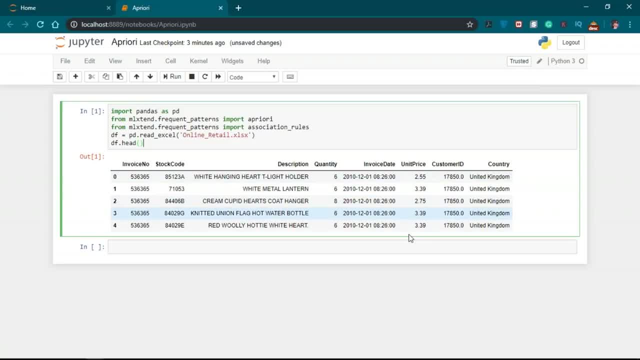 stock code, the description, the quantity, the invoice data, unit price, customer id and the country. now, next in this step, what we're going to do is do data cleanup, which includes removing the spaces from some of the descriptions, and drop the rules that do not have invoice numbers and remove the credit card transactions, because that is of no use to us. 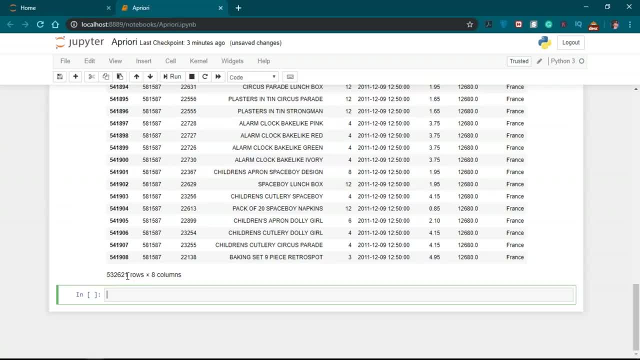 so, as you can see here the output in which we have like 532 000 rows with eight columns. so after the cleanup, we need to consolidate the items into one transaction per row with each product for the sake of keeping the data set small. we are only looking at the sales for france. 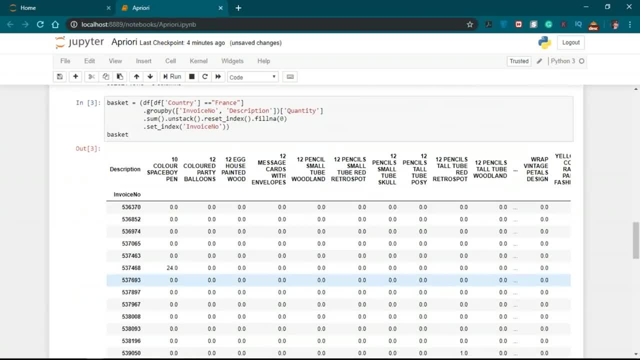 so, as you can see here, we have excluded all the other sales. we are just looking at the sales for france now. there are a lot of zeros in the data, but we also need to make sure any positive values are converted to one and anything less than zero is set to zero. so, as you can see, here we are still. 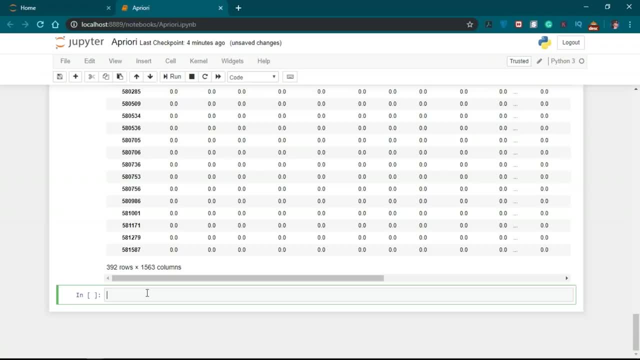 392 rows. we're gonna encode it and see check again. now that you have structured the data properly, let's go on and take a look at the data in france. in this step, what we're going to do is generate frequent item sets that have support, at least. 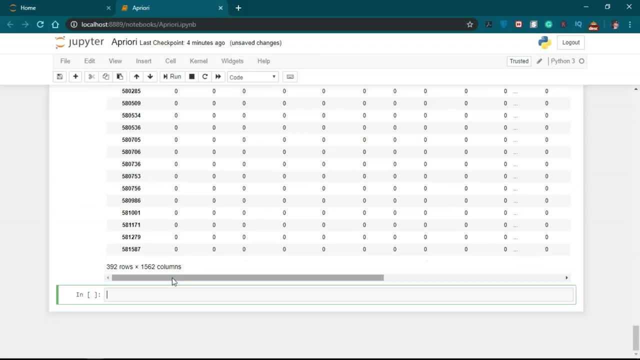 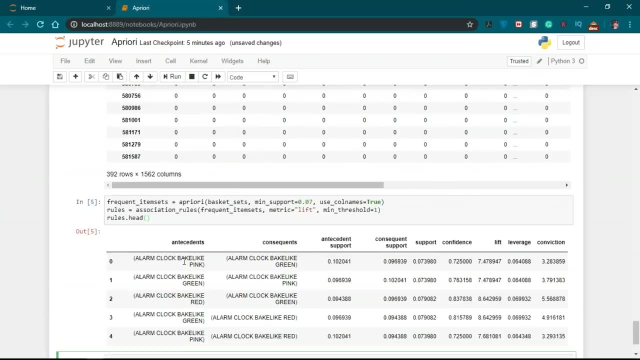 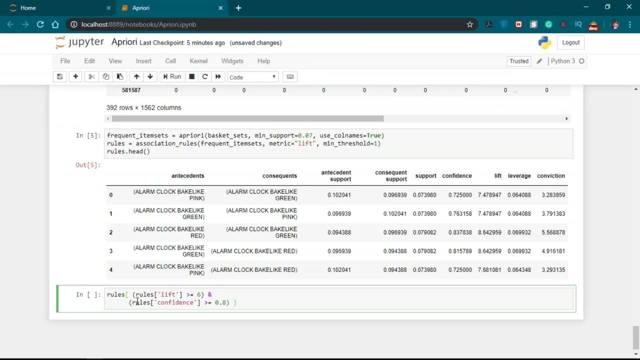 seven percent. now, this number is chosen so that you can get close enough and generate the rules with the corresponding support, confidence and lift. so again, as you can see here, the minimum support is 0.7. now what if we add another constraint on the rules, such as the lift is? 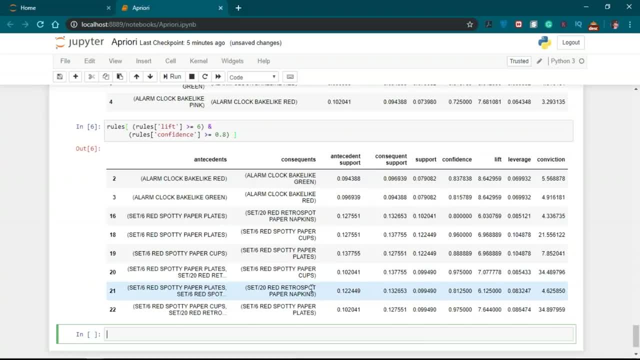 greater than 6 and the confidence is greater than 0.8. so, as you can see, here we have the left hand side, on the right hand side of the association rule, which is the antecedent and the consequence, we have the support, we have the confidence, the lift, the leverage and the conviction. 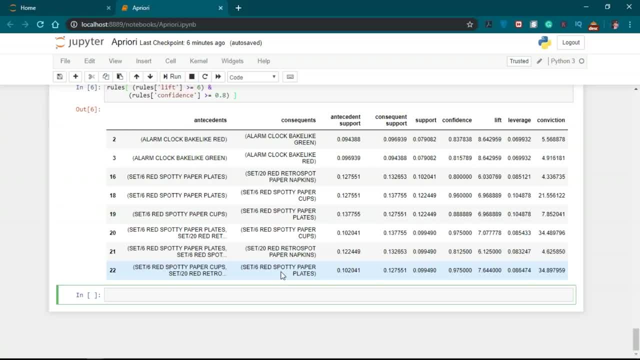 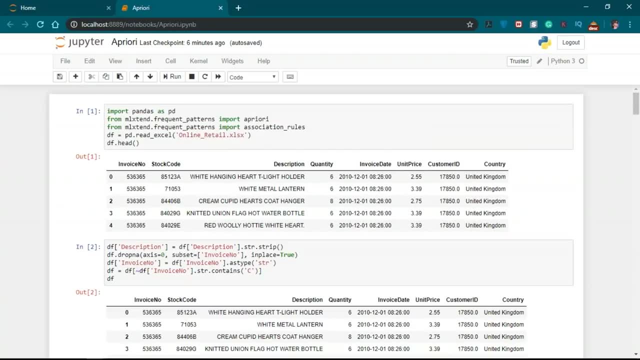 so, guys, that's it for this session. that is how you create association rules using the a priori algorithm, which helps a lot in the marketing business. it runs on the principle of market basket analysis, which is exactly what we're going to do in this step. so we're going to. 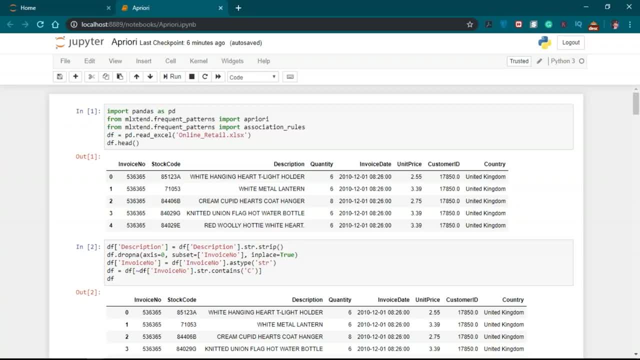 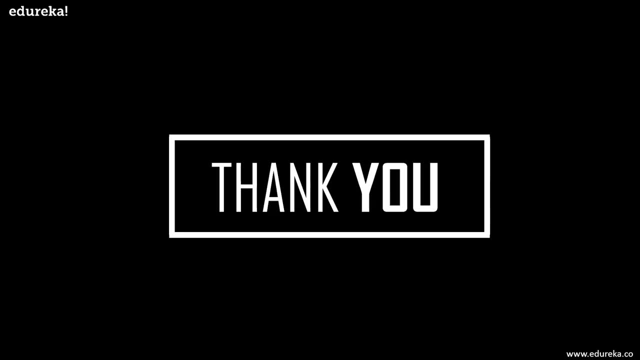 create association rules using the a priori algorithm, which is exactly what big companies like walmart, you have, reliance and target 2. even ikea does it, and i hope you got to know what exactly is association rule mining, what is lift confidence and support and how to create. 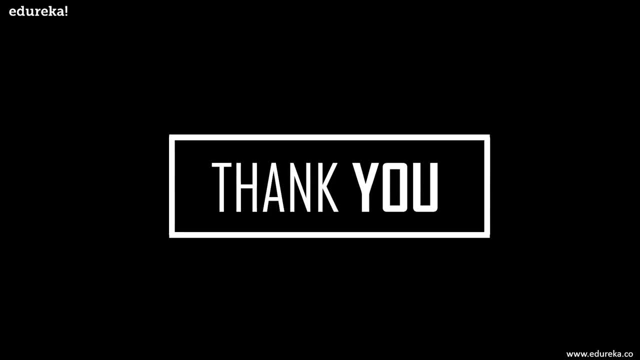 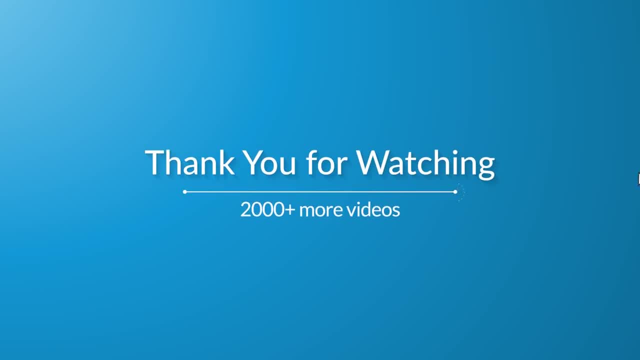 association rules. that we have any queries, feel free to mention it in the comment section below. till then, thank you and happy learning. i hope you have enjoyed listening to this video. please be kind enough to like it and you can comment any of your doubts in the comment section below.